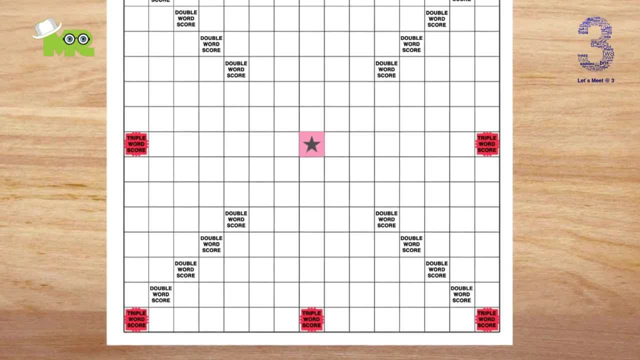 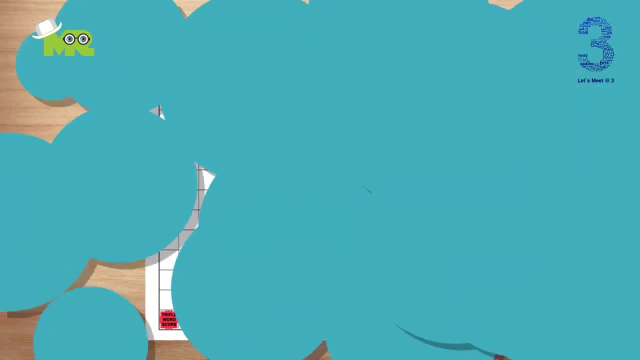 How to make your own Scrabble board game. Repeat this process to the remaining three corners, like here: How to make your own Scrabble board game. Now, color pink: all of the double word score spots, like in this way: How to make your own Scrabble board game. 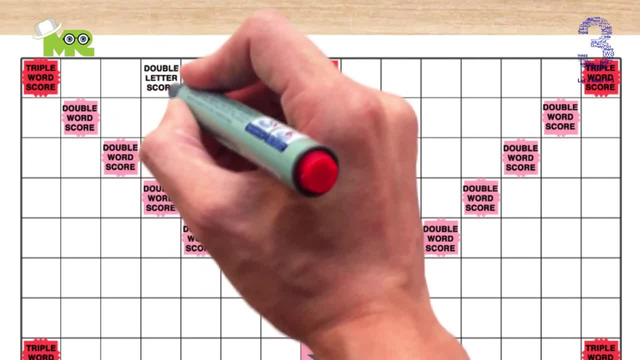 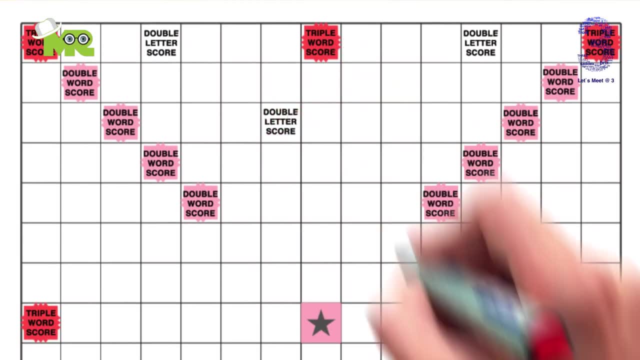 Double letter score. How to make your own Scrabble board game In row one, square four and twelve: write double letter score like so: How to make your own Scrabble board game In row three, square seven and nine: write double letter score like this: 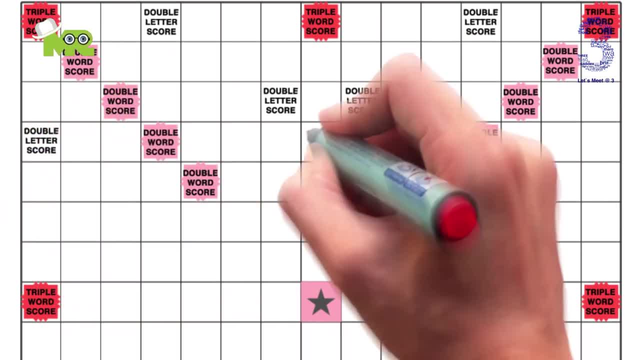 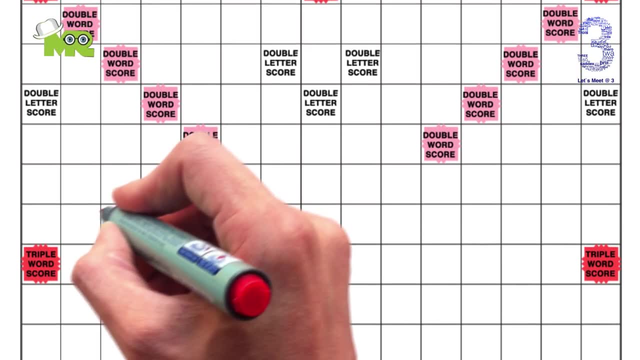 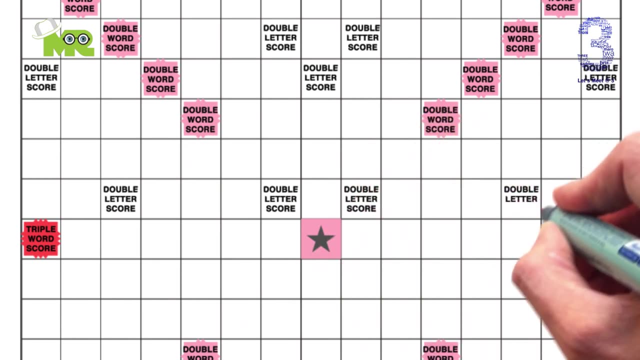 How to make your own Scrabble board game In row four, square one. eight and fifteen: write double letter score like this: How to make your own Scrabble board game In row seven, square three. seven, nine and thirteen: write double letter score like this: 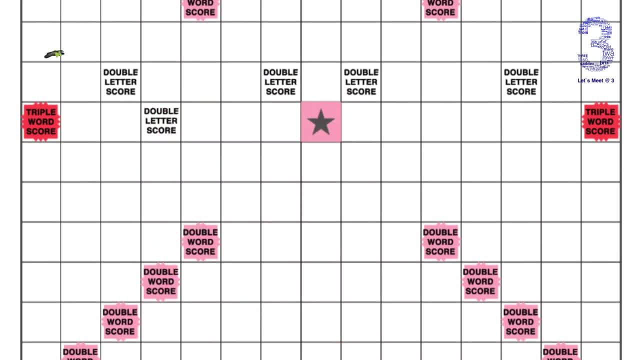 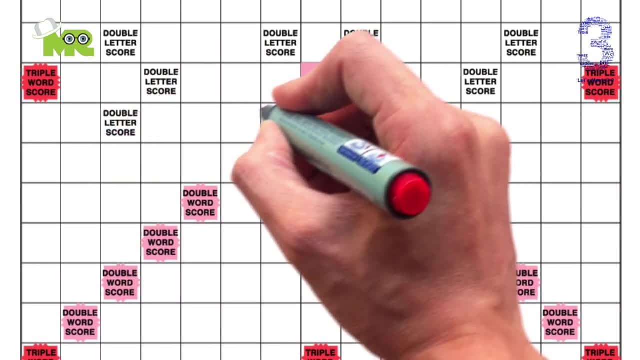 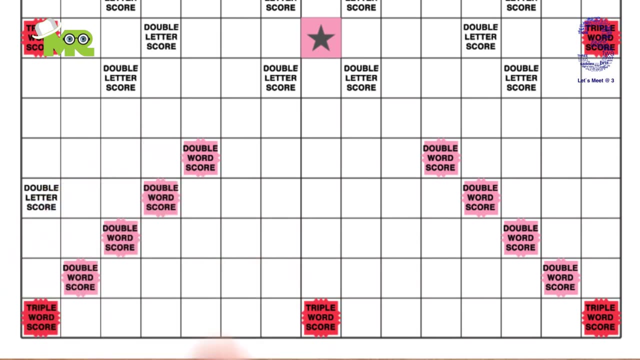 How to make your own Scrabble board game. In row eight, square four and twelve, write double letter score like this: in row 9, square 3, 7, 9 and 13: write double letter score like this in row 12, square 1, 8 and 15: write. 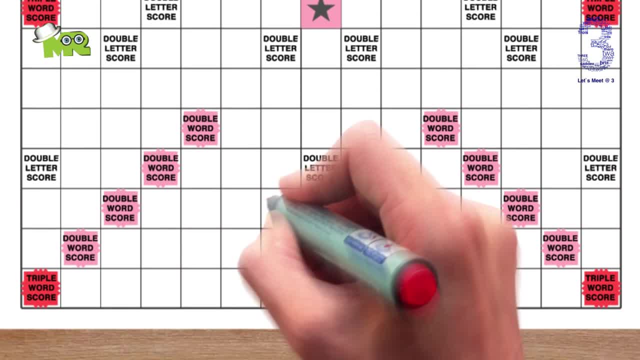 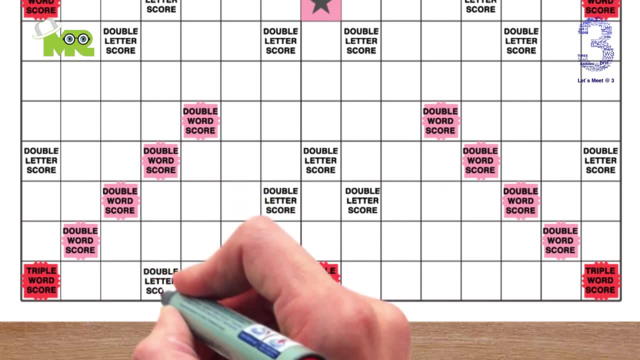 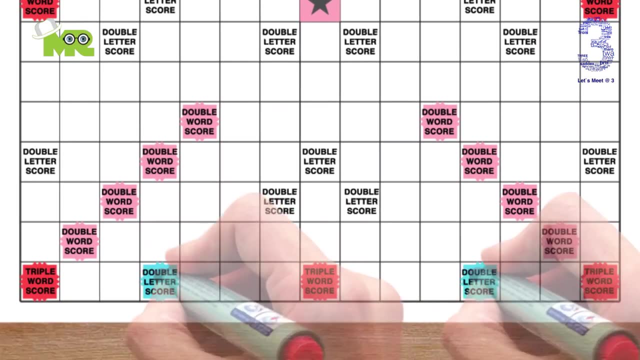 double letter score like this: in row 13, square 7 and 9: write double letter score like so: in row 15, square 4 and 12: write double letter score like so: this is how it should look when it's all said and done now. color: light blue. all of the double letter score spots like in this way: triple letter. 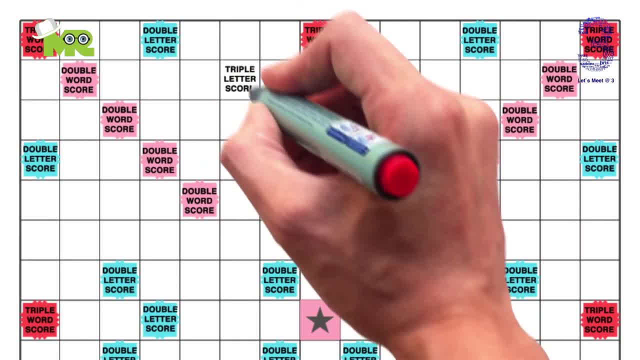 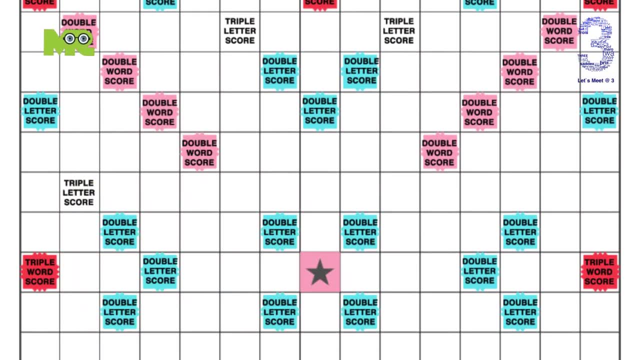 score in row 2, square 6 and 10: write triple letter score like this. in row 6, square 2: 6, 10 and 14: write triple letter score just like this now in Row 10, square 2: 6, 10 and 14 write: 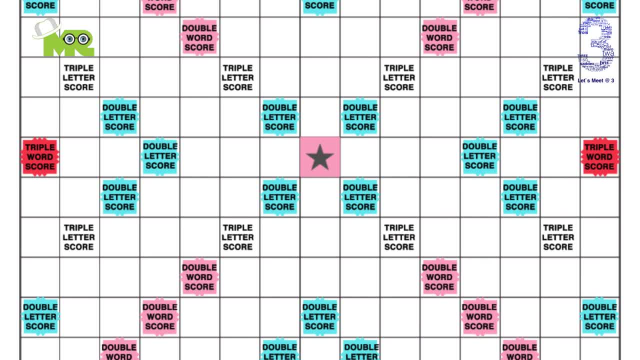 triple letter score. next, row 7 and 10: write double letter score like so: in row 8: F dollar, middle 11 of the sweetاه school year. here's how it should look when you have double letter score. triple letter score like this: in row 14, square 6 and 10: write triple letter score like this: 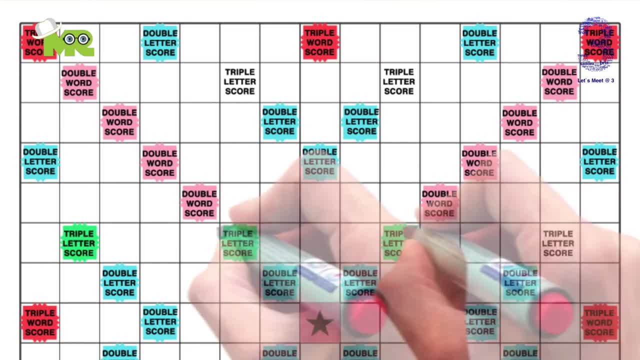 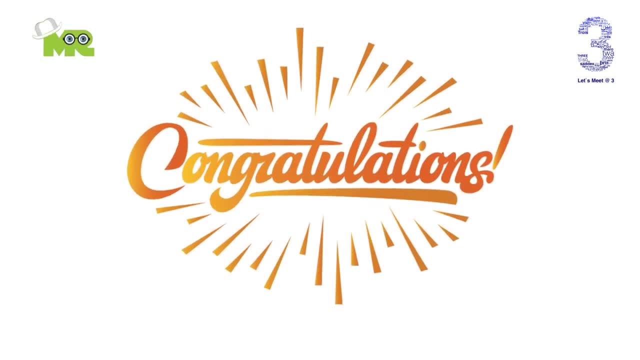 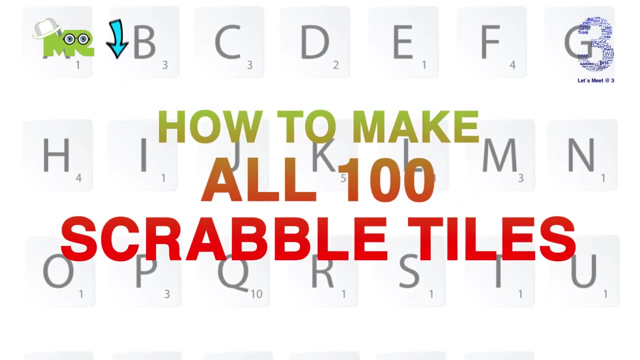 now color light green in all the double letter score spots. it should look like this when it's done: congratulations, you've just created your own scrabble board game. have fun, friends. if you would like to learn how to make all 100 scrabble tiles, please click here or click the link in the